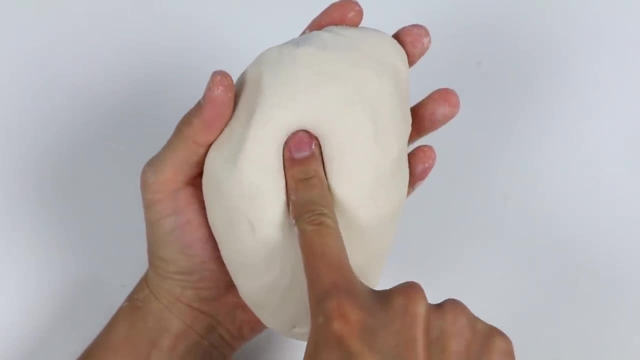 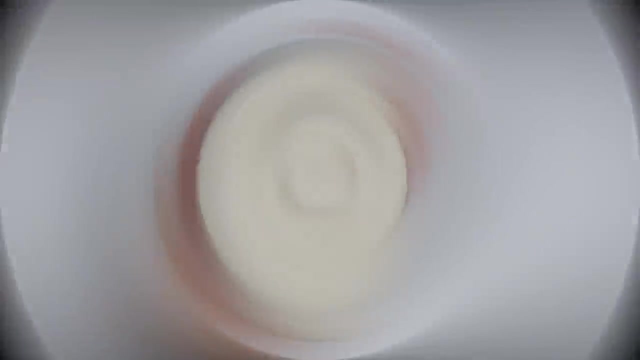 Alright and we're finished. Check out our homemade Play-Doh. I can't wait to make some shapes with this, But before we do that, we should color our dough first. Let me roll this out a bit and then separate the dough into three pieces. 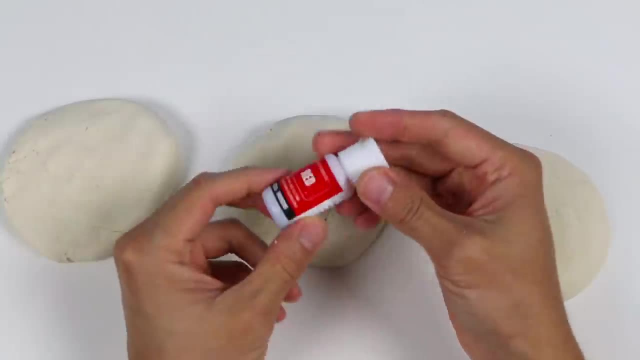 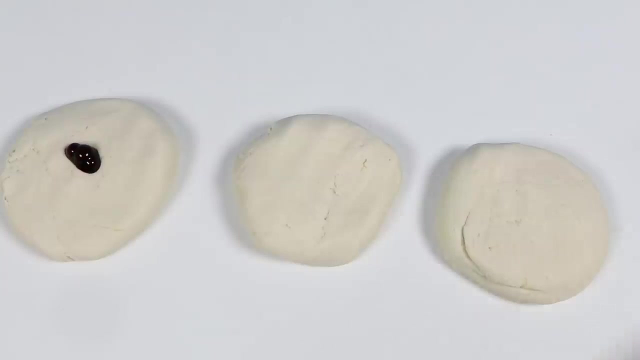 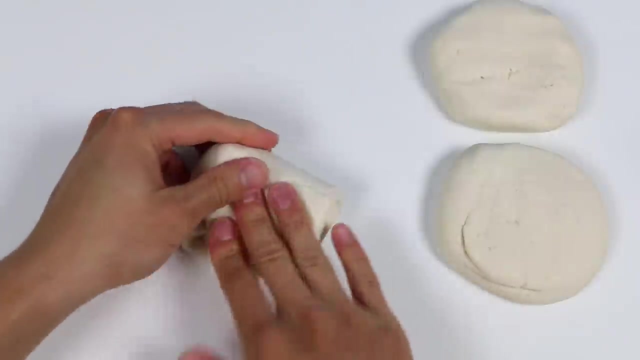 There we go. These look pretty even. Let's make one of our doughs red. Now let's mix our dough up. Start by folding it and then just knead the dough until it turns red. Simple as that. Now, if you don't want your hands to stain, use gloves during this part. 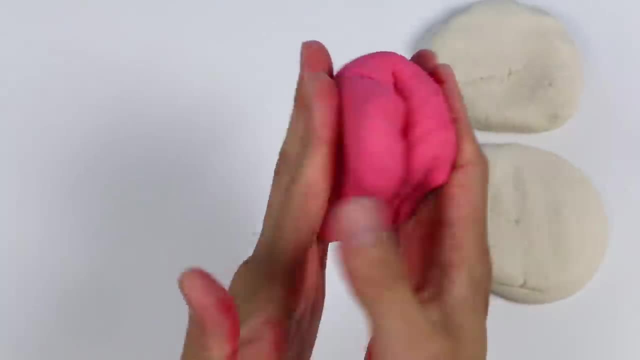 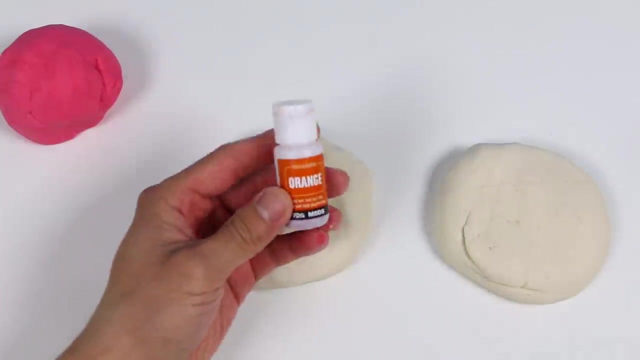 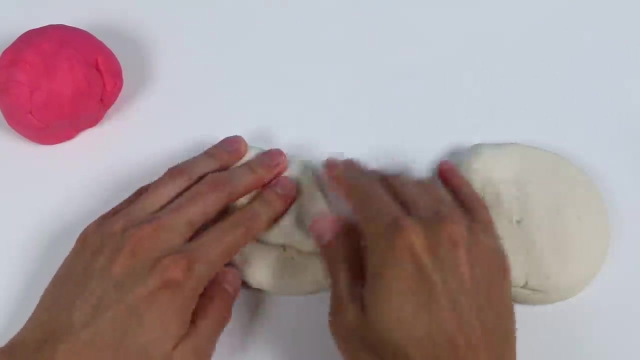 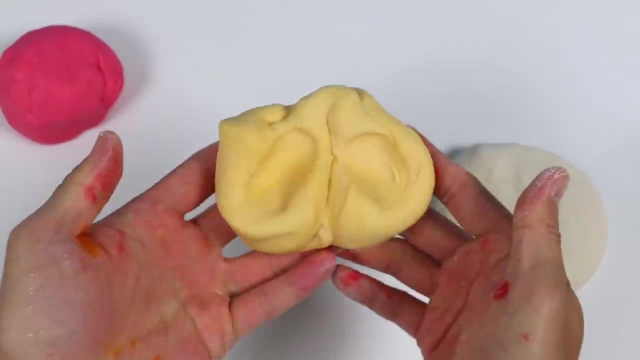 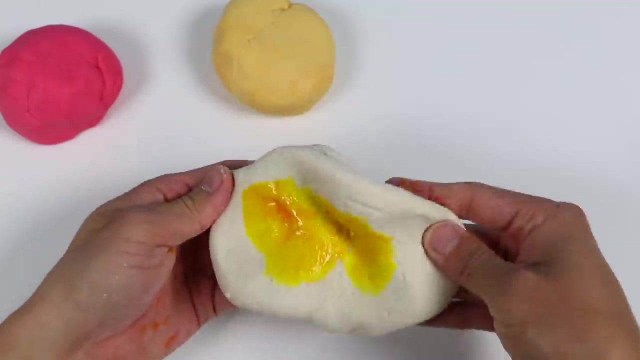 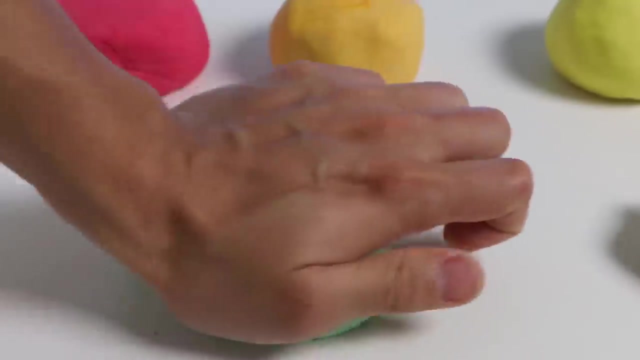 Okay. so here's a closer look at our red edible Play-Doh. Now let's make orange Knead- this Awesome. Here's our orange dough. Now let's make yellow Perfect. I went ahead and made some more dough to make a few more colors. 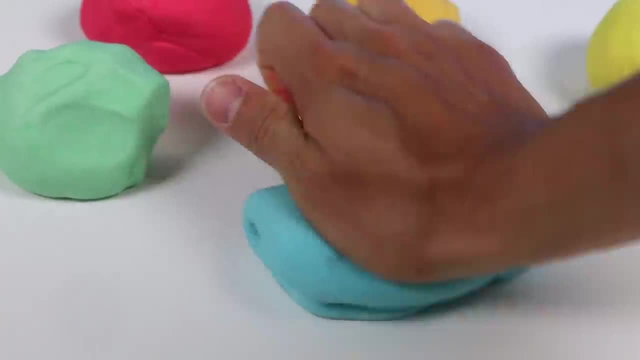 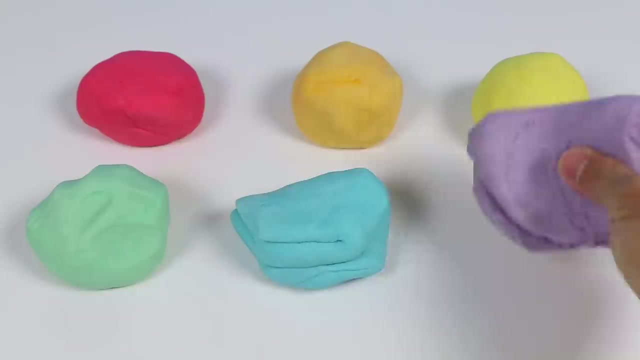 Here's green, Here's blue, Here's purple. With these six colors, we should be able to make some pretty awesome stuff. Okay, let's start by using some of this red dough. Okay, let's start by using some of this red dough. 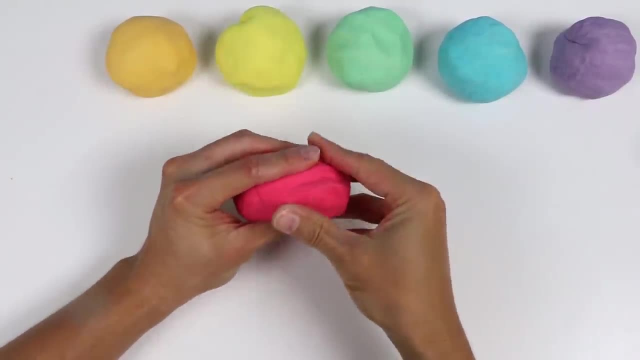 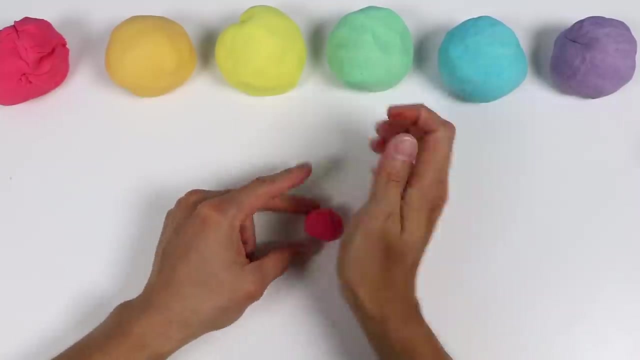 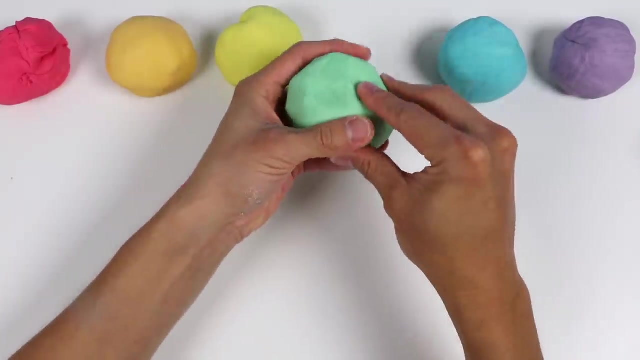 Oh my gosh, it really feels like I'm playing with Play-Doh. Let me shape this into a strawberry. Now. let's press this into our big dough and shape it into a real strawberry. Perfect, grab some green dough to make strawberry leaves. roll it out. these colors are lighter than actual. 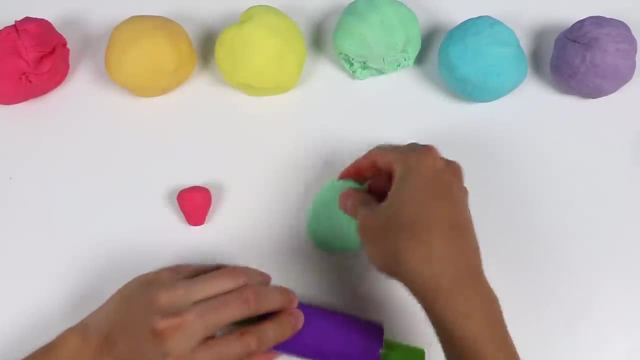 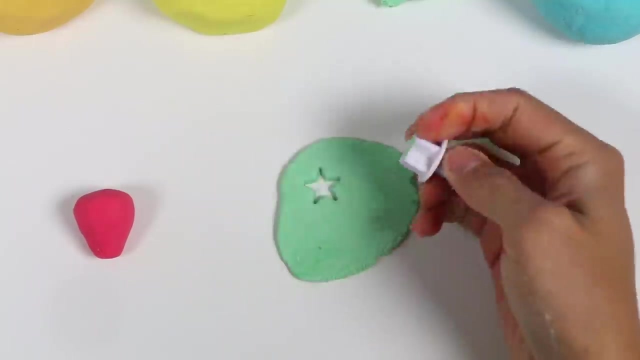 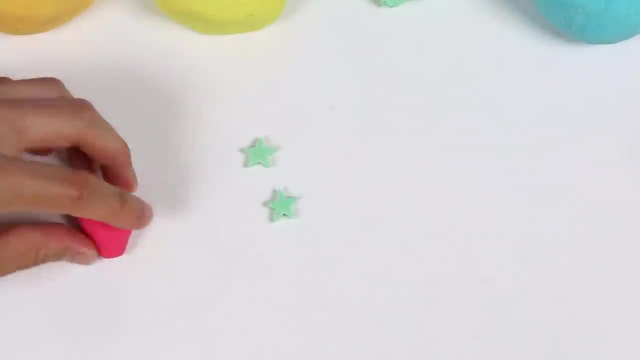 play-doh, but besides that, everything else looks and feels similar. guess, we'll see if there's any more differences as we keep playing with them, but so far, so good. now let me use this star stamp. stamp out a couple stars. okay, now let's add a bunch of details to our strawberry poke- a bunch. 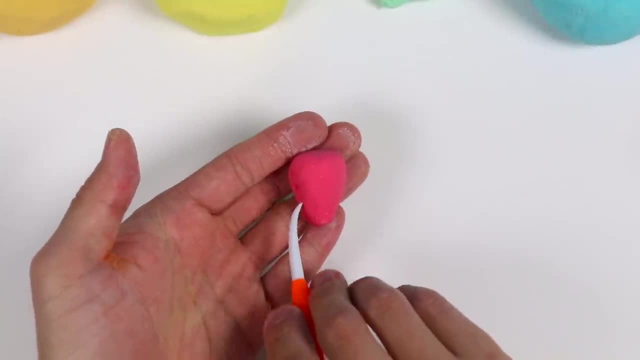 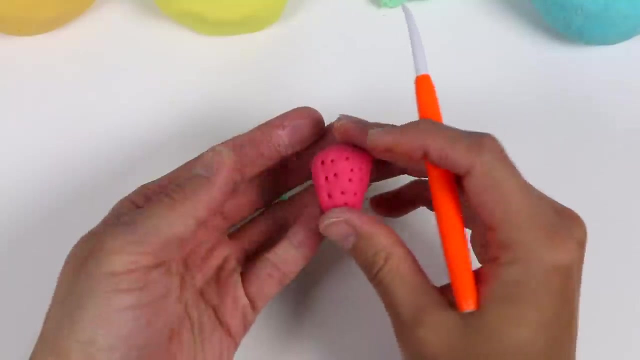 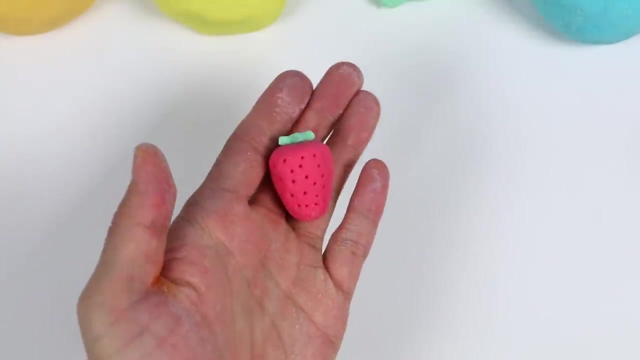 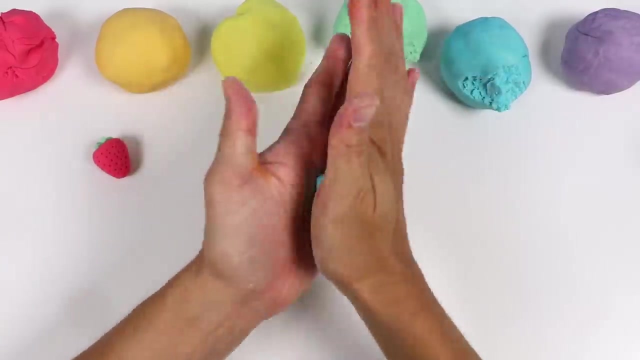 of holes- awesome. now let's attach one of the leaves on top. here's a closer look at our strawberry. okay, let's make another fruit using this blue dough. we'll make a blueberry, so let's make a round shape. that looks good. now let's attach the blueberry leaves. 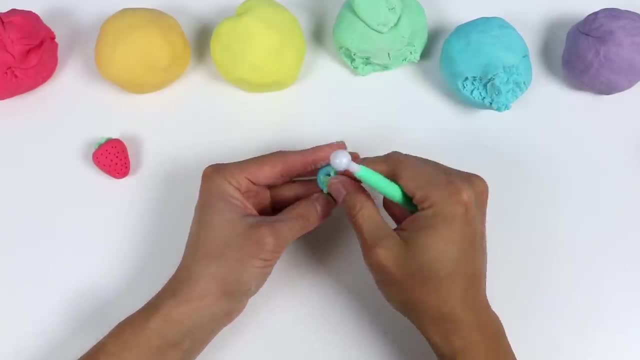 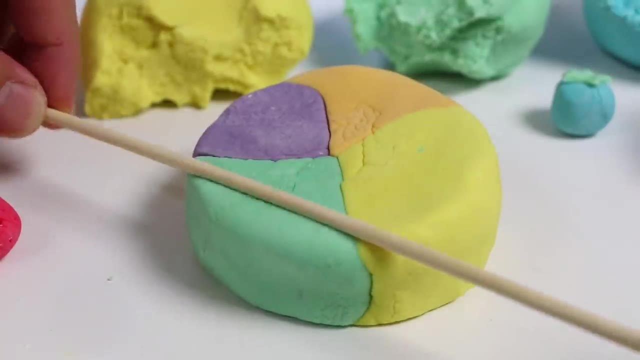 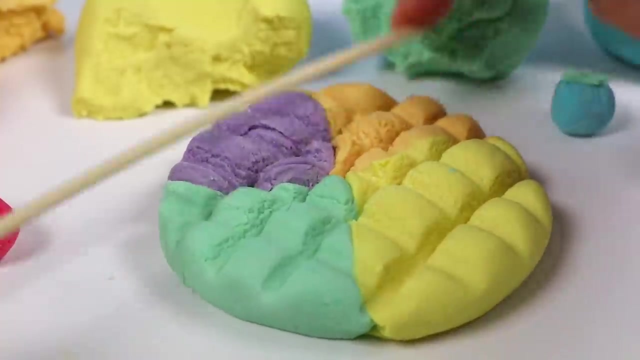 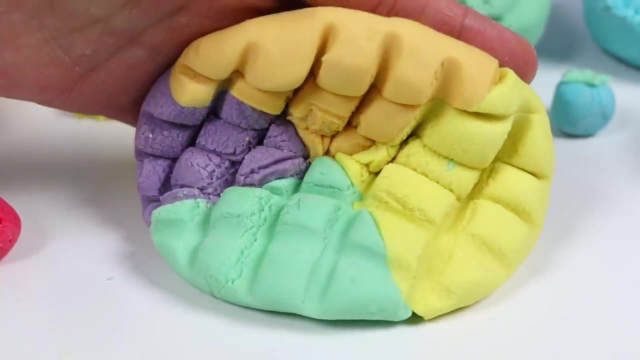 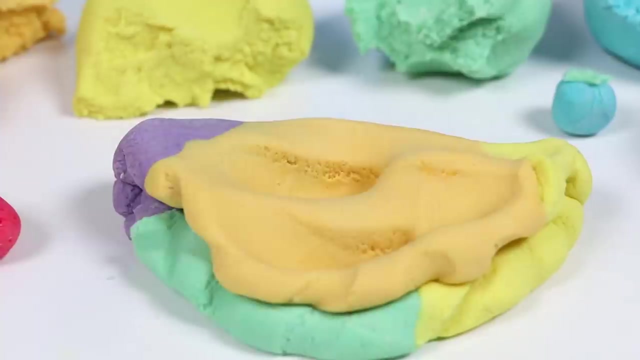 poke a hole. awesome. here's a closer look at our blueberry. okay, so I combined green, purple, orange and yellow. now let's use the skewer stick to make a waffle design. now let's fold our fluffy waffle. look at that. so, so all right. now let's just play with this for a bit. so I know, I said this is edible play-doh. 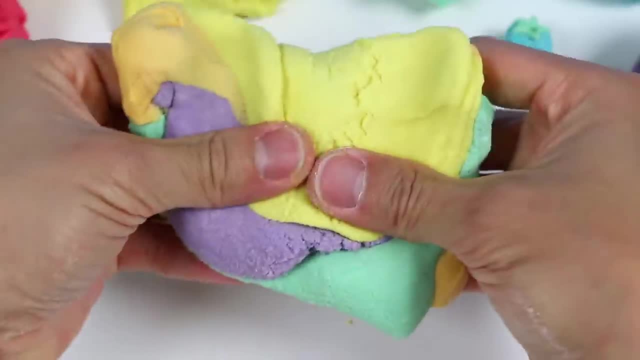 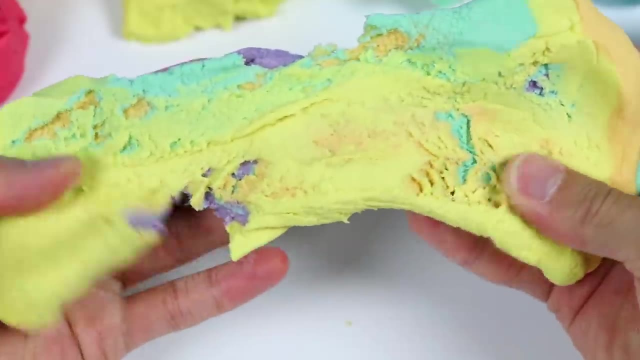 but compared to the marshmallow one, this one definitely won't taste as good. this was made as a substitute to play-doh, so taste wasn't a high priority and as I was playing with this, compared to actual play-doh, this is much softer and stretchier, but it's nice that we can. 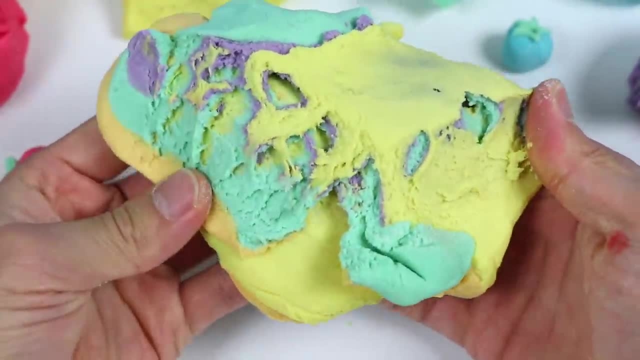 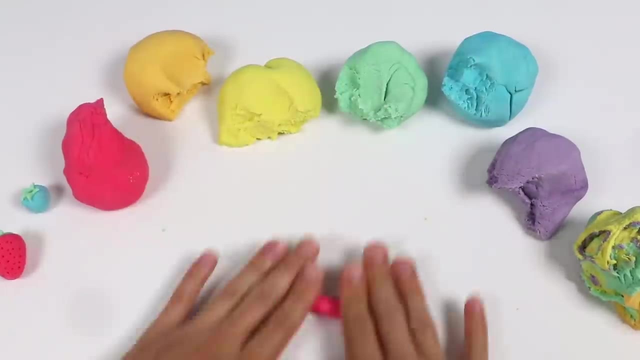 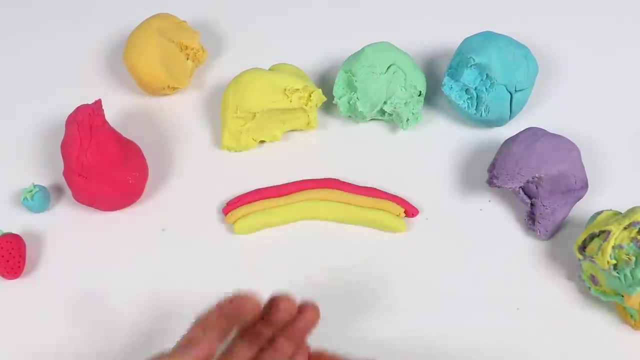 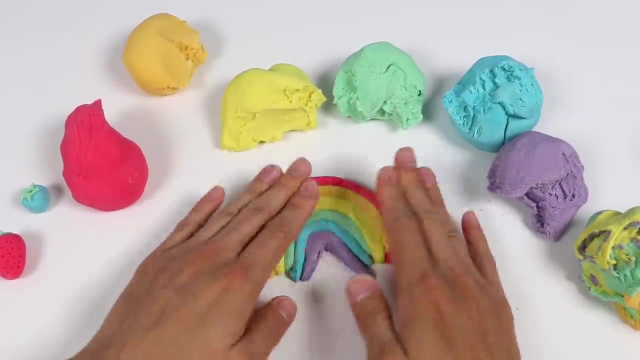 still make all of the shapes we want. all right now let's use our dough to make a rainbow. give me a minute while I make all of the shapes with each color. there we go now. let's make the rainbow shape now. let's clean this up a bit awesome. here's a closer. 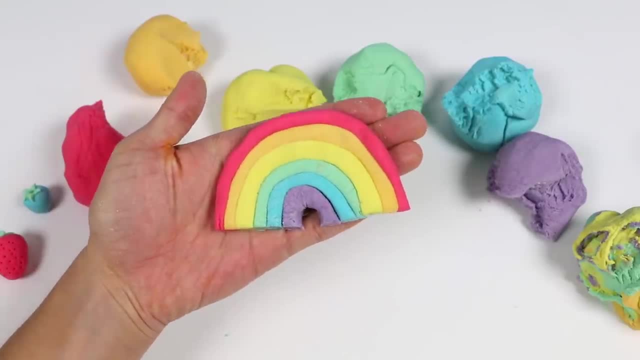 look at our homemade rainbow play-doh. do you like this version better or the actual play-doh version? now? if you watch our channel, you know that we've been doing it for a while now, so if you're interested in the rainbow play-doh, feel free to let us know in the comments down below. 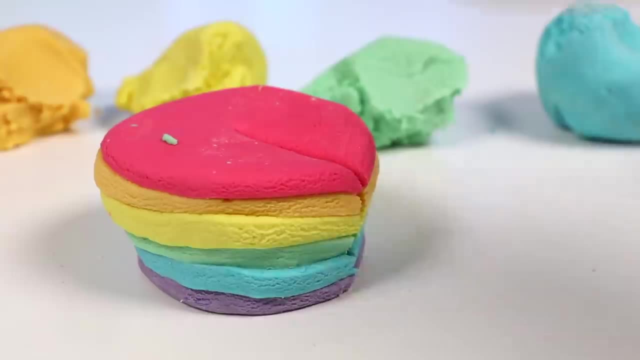 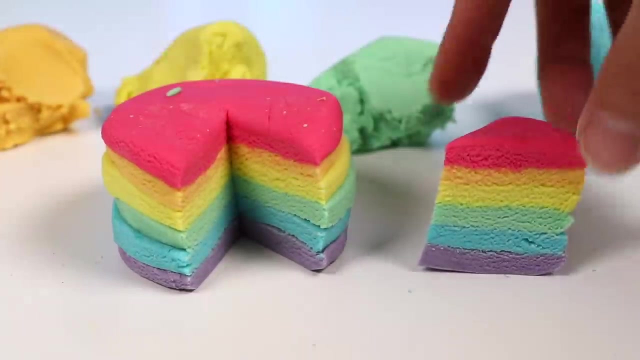 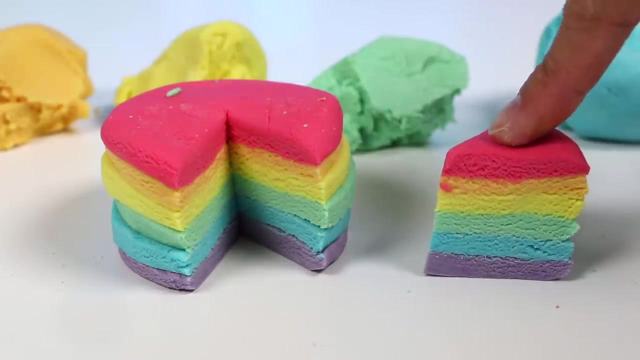 we love to make play-doh cakes, So here's a six-layered cake. Let's slice this up. Ooh, looks pretty similar. You know, since this is edible, this might actually be good if we bake it in the oven. Might need to tweak it a little bit. create a nice sweet glaze with fruit toppings.